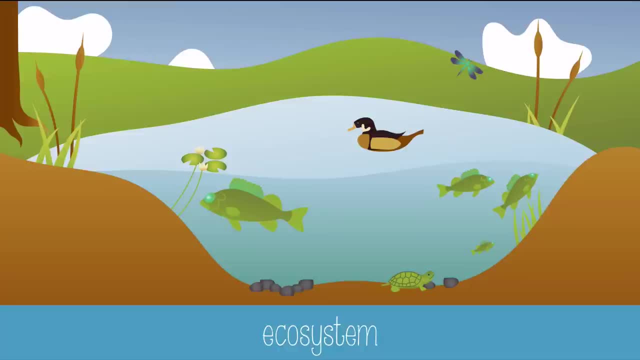 organisms interact in ways that affect their survival. For instance, insects and fish eat aquatic plants and the turtles eat the fish. The non-living, or physical and chemical things include the chemical composition of the pond, its pH, its levels of dissolved oxygen and carbon. 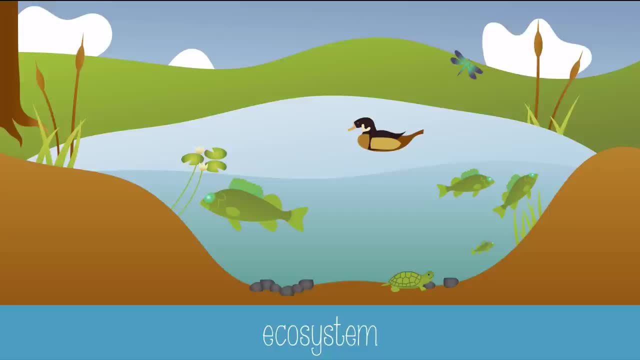 dioxide and its supply of nitrogen, which all help to determine what kinds of organisms live in the pond and how abundant they are. The non-living, or physical and chemical things include the chemical composition of the pond, its pH, its level of nitrogen, which all help to determine. 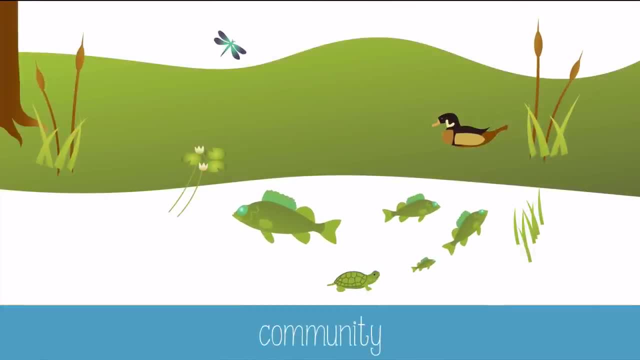 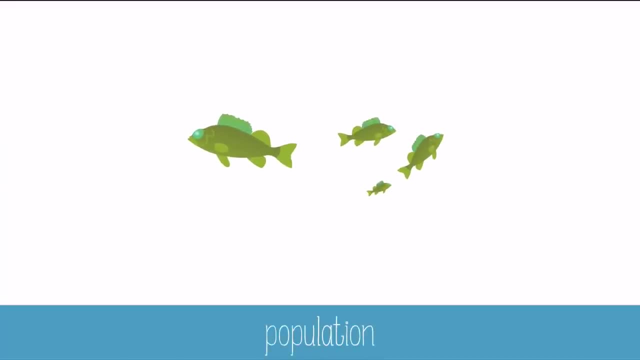 what kinds of organisms live in the pond and how abundant they are. A community is all of the interacting organisms in an area. It does not include the non-living factors. A population is all of the organisms of one type of species in the area, and an organism refers to an individual. 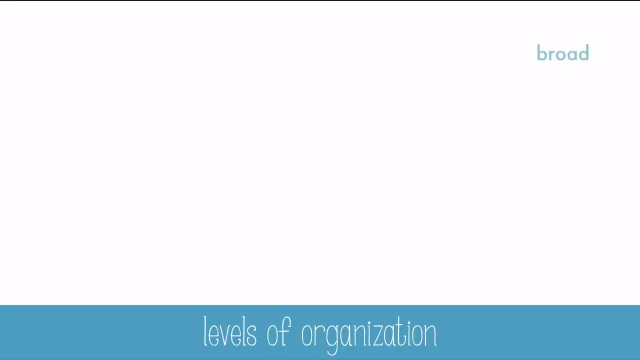 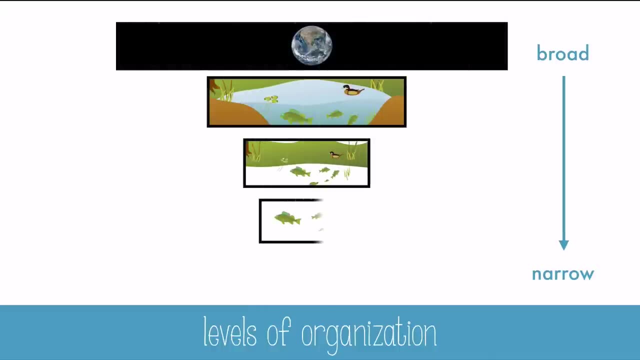 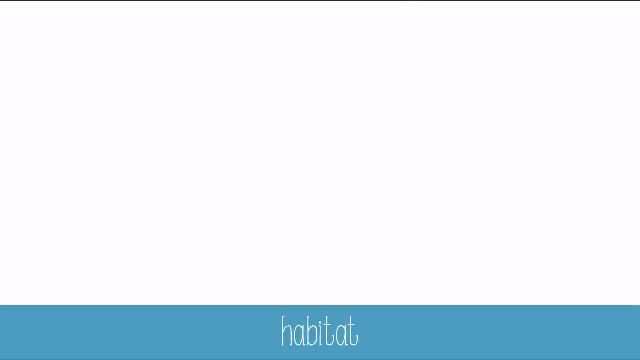 animal. In order, the levels of organization from the most broad to the narrowest are the biosphere, ecosystem, community, population and organism. When we talk about organisms, we talk about where an organism lives, Instead of saying ecosystem, which might still be a fairly 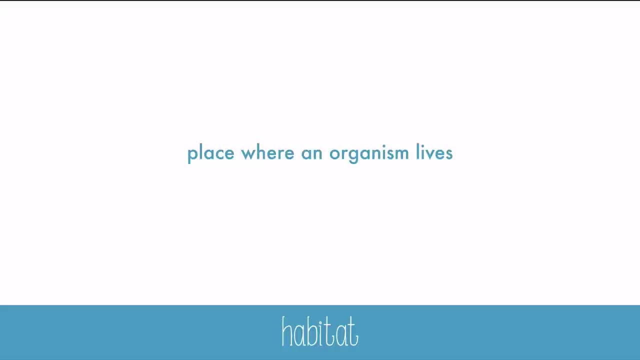 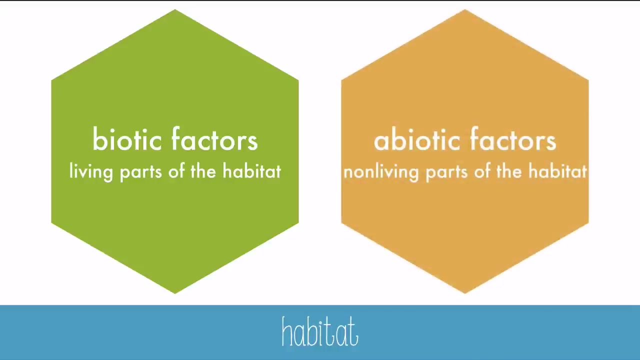 large area, we could talk about its habitat. It's just a word that means the place where an organism lives. A habitat includes both biotic and abiotic factors. Biotic factors are the living parts of the habitat and when you add the letter A in front of the word, it means not living, so abiotic. 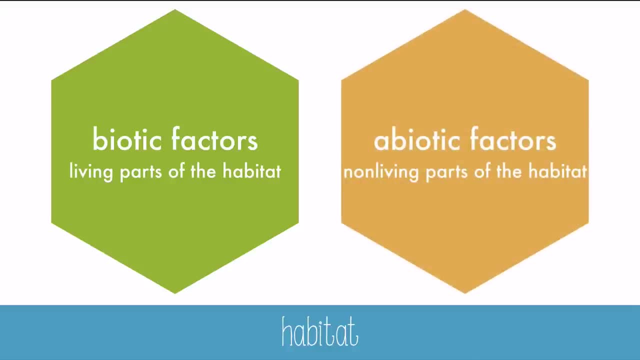 factors are the non-living parts of the habitat, Using the pond ecosystem as an example. biotic factors include grasses, algae, fish, birds and animals. The non-living or physical and chemical factors include birds and insects. The abiotic factors include the pH of the water, rocks, soil. 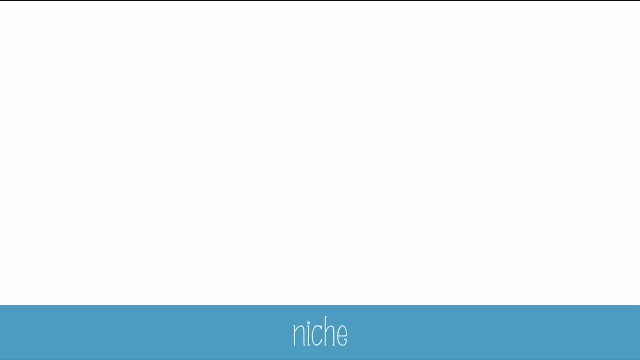 the sunlight and temperature. Now you may sometimes hear people try to use the word habitat and the word niche interchangeably, and that's not quite how they should be used. A niche is the job or role of the organism within its environment, So habitat is a home and niche is 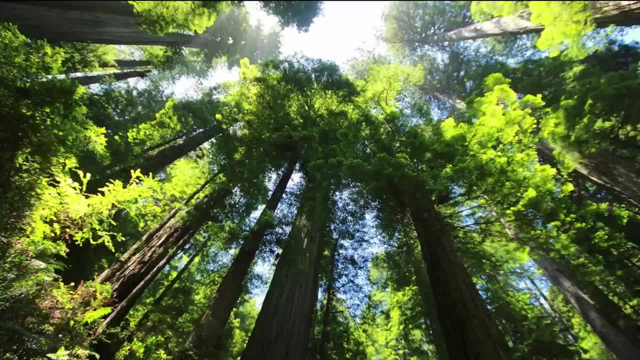 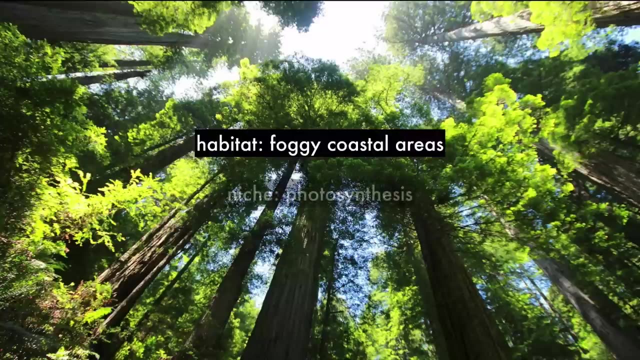 a job. For example, a redwood tree takes energy from the sun and turns it into sugar using photosynthesis. Redwood trees are often found in foggy coastal areas like Santa Cruz, California. The habitat is the foggy coastal areas like California and the niche is converting the sun's energy into sugar by photosynthesis. 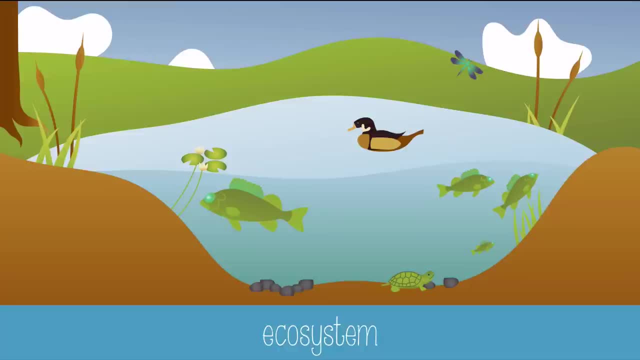 organisms interact in ways that affect their survival. For instance, insects and fish eat aquatic plants and the turtles eat the fish. The non-living, or physical and chemical things include the chemical composition of the pond, its pH, its levels of dissolved oxygen and carbon. 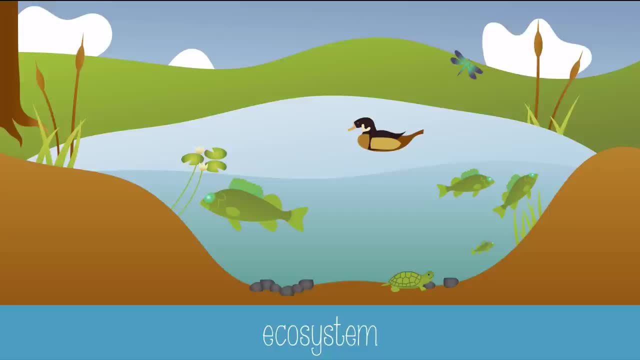 dioxide and its supply of nitrogen, which all help to determine what kinds of organisms live in the pond and how abundant they are. The non-living, or physical and chemical things include the chemical composition of the pond, its pH, its level of nitrogen, which all help to determine. 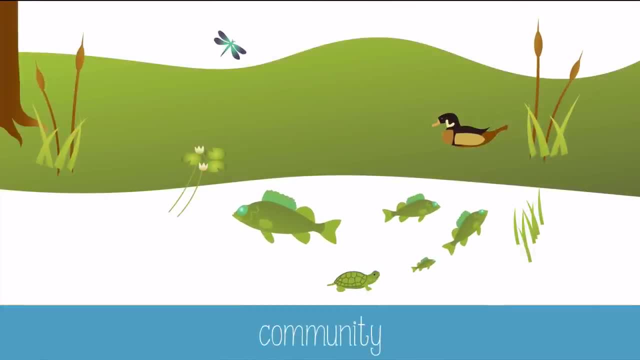 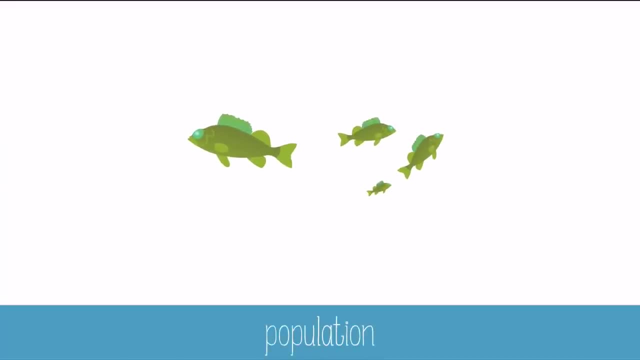 what kinds of organisms live in the pond and how abundant they are. A community is all of the interacting organisms in an area. It does not include the non-living factors. A population is all of the organisms of one type of species in the area, and an organism refers to an individual. 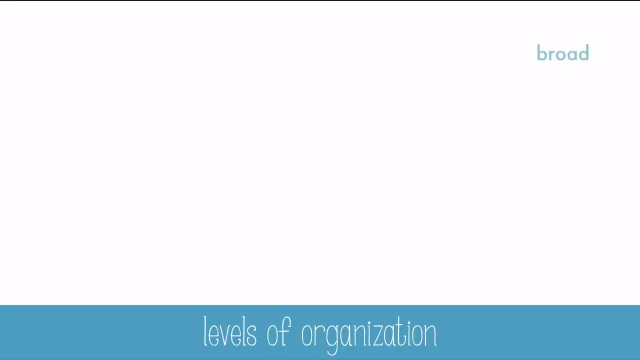 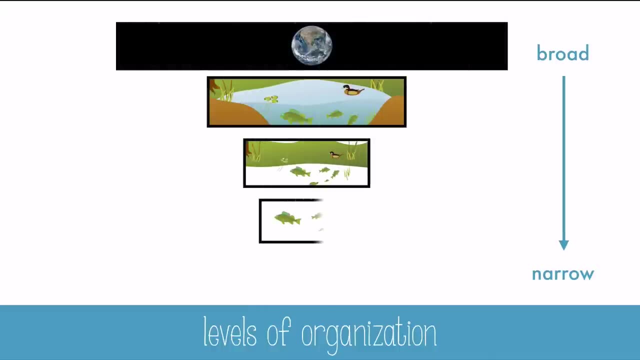 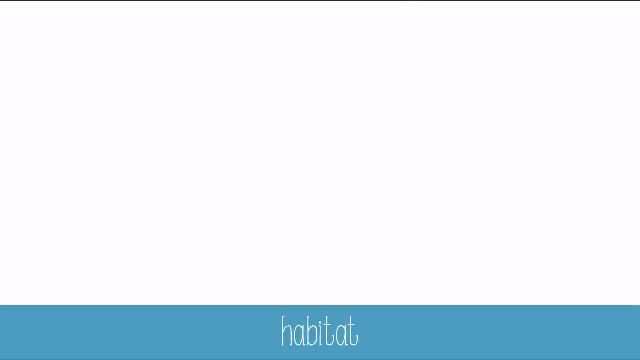 animal. In order, the levels of organization from the most broad to the narrowest are the biosphere, ecosystem, community, population and organism. When we talk about organisms, we talk about where an organism lives, Instead of saying ecosystem, which might still be a fairly 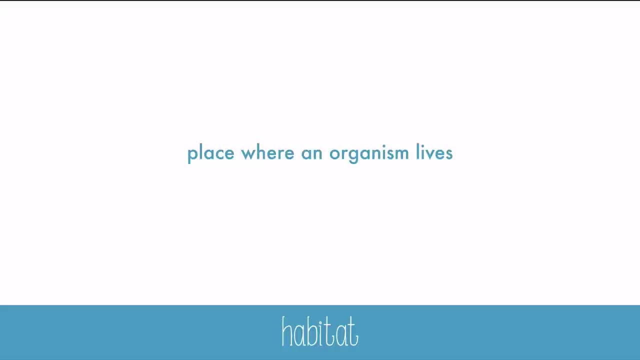 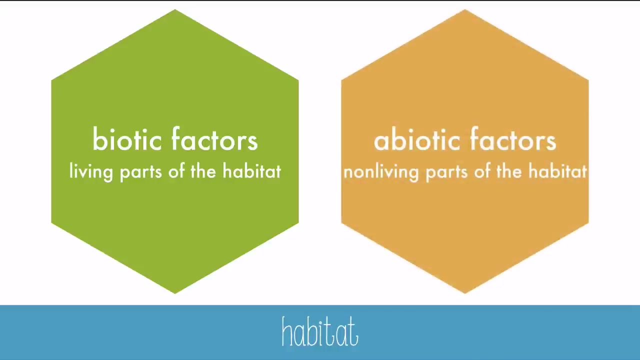 large area, we could talk about its habitat. It's just a word that means the place where an organism lives. A habitat includes both biotic and abiotic factors. Biotic factors are the living parts of the habitat and when you add the letter A in front of the word, it means not living, so abiotic. 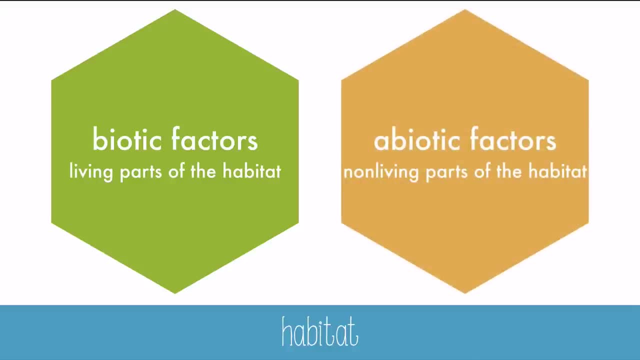 factors are the non-living parts of the habitat, Using the pond ecosystem as an example. biotic factors include grasses, algae, fish, birds and animals. The non-living or physical and chemical factors include birds and insects. The abiotic factors include the pH of the water, rocks, soil. 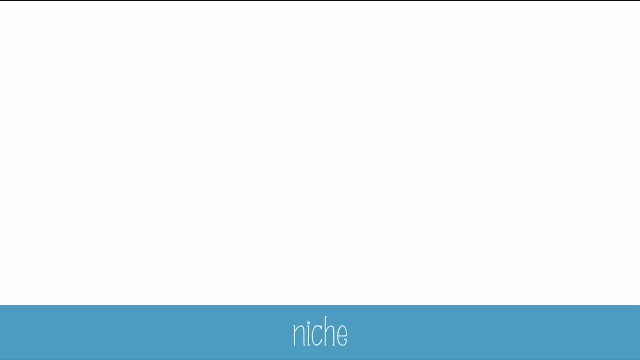 the sunlight and temperature. Now you may sometimes hear people try to use the word habitat and the word niche interchangeably, and that's not quite how they should be used. A niche is the job or role of the organism within its environment, So habitat is a home and niche is 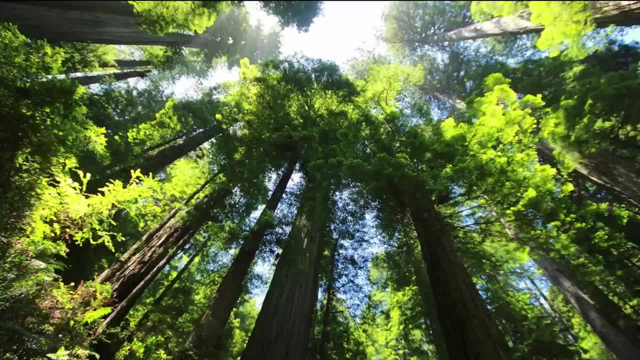 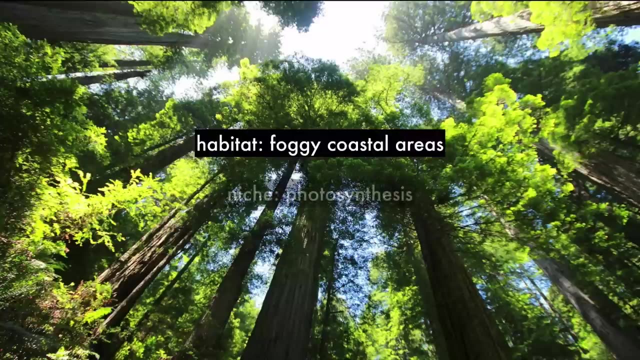 a job. For example, a redwood tree takes energy from the sun and turns it into sugar using photosynthesis. Redwood trees are often found in foggy coastal areas like Santa Cruz, California. The habitat is the foggy coastal areas like California and the niche is converting the sun's energy into sugar by photosynthesis.